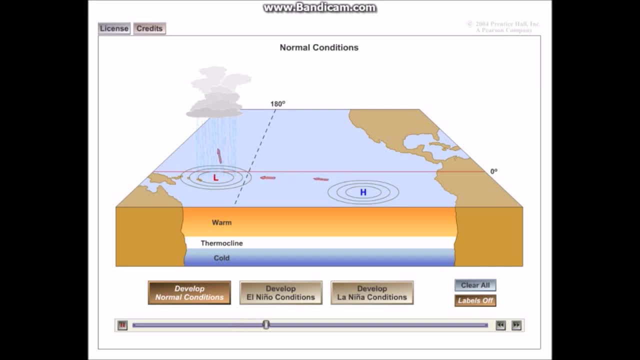 falls in this area and, as a cell, completes and it moves around. the cooler air over the coast of South America sinks and this causes this circular movement of air, which we call the Walker cell. It is this cell that generates the normal weather and oceanic conditions that we have in the Pacific region Now. 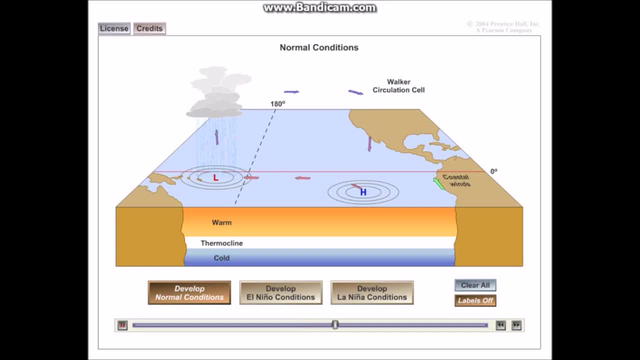 these trade winds that move from the coast of South America to the coast of Southeast Asia. what they do is they also drag water with it, and they tend to move this water and make the sea level even slightly higher in the Southeast Asian coast than it is in the South American coast. Eventually, what will occur is also: 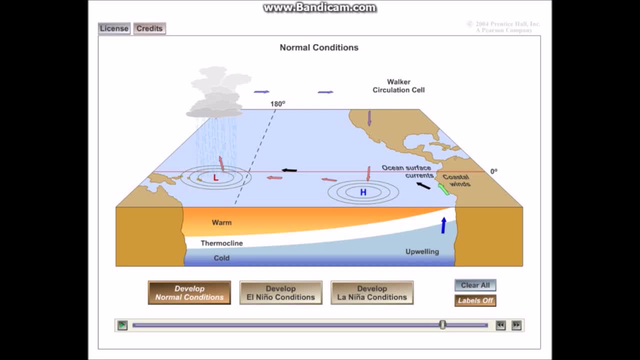 it will cause this cold upwelling of water that you have on the South American coast. that is fantastic for fish and is why the Chilean and the Peruvians are have very large fishing industries, So normal conditions imply that you have the Walker cell. the trade winds are blowing from the coast. 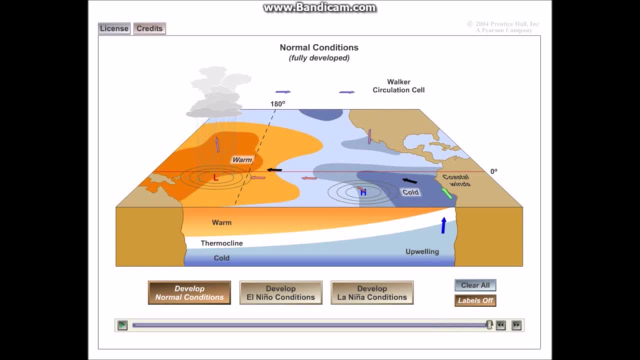 of South America to the coast of Southeast Asia. the sea level is slightly higher in Southeast Asia than it is in South America and you get this large body of warm pooling water in Southeast Asia and you get this cold body of water caused by upwelling and maybe the Peruvian 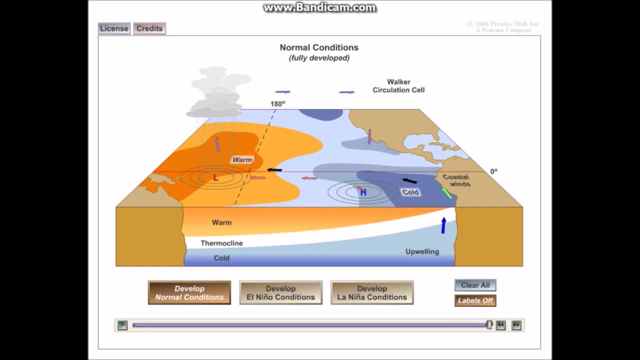 current, that is, in South America, and these are the normal conditions that occur Now. what occurs in El Niño conditions or in Elso conditions is that the trade winds that are blowing from the coast of South America to the coast of Southeast Asia break down. They become less and less and weaker, and when 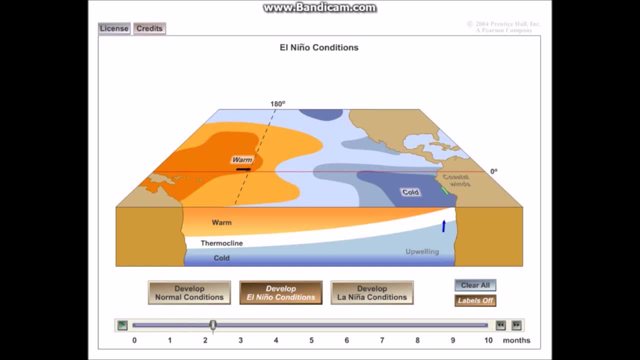 eventually they do break down. as you can see over here, this cold or the cold water and the warm water are no longer held in place by these surface currents, so the warm water tends to slow down and the cold water tends to slow down and the slosh back, it tends to move back towards the coast of South America. and 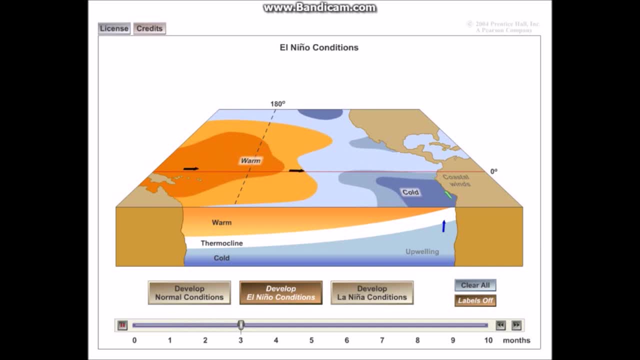 with it. obviously it brings all of the warmth that it had with it and it pushes back this cold water, as you can see over there, and that upwelling that was going on begins to decline. the thermocline sinks back down to its normal previous levels. So, as you can see over here, the now warm water has spread all the way. 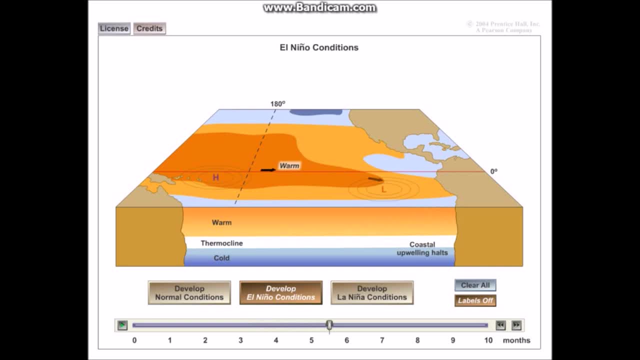 across the Pacific Ocean and is now knocking on the doors of California and, you know, Chile and Peru. Now, because of this change, even though you can see on this diagram that it appears to be quite warm in Southeast Asia- and this is not as warm as it would- 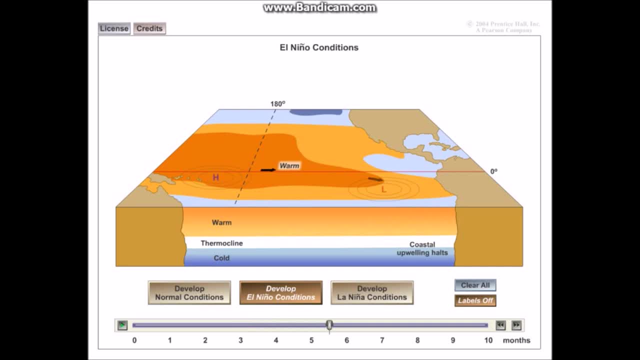 have been otherwise. so if you look at sea surface temperature maps, you would actually see a slight decline in temperature in that region. Now what occurs is that you have this element that we call the oscillation, or southern oscillation is why El Niño conditions are sometimes referred to as 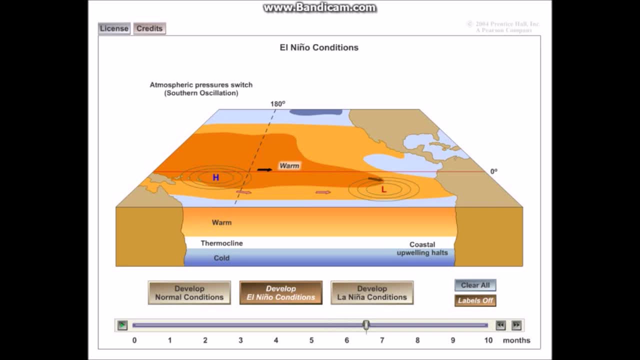 Enso conditions: El Niño, Southern Oscillation. So the Walker cell that previously existed under normal conditions completely broke down and, as you can see from the high and the low pressure, has now reversed. High pressure is found over the coast of Southeast Asia rather than the coast of South America, and what this causes is it. 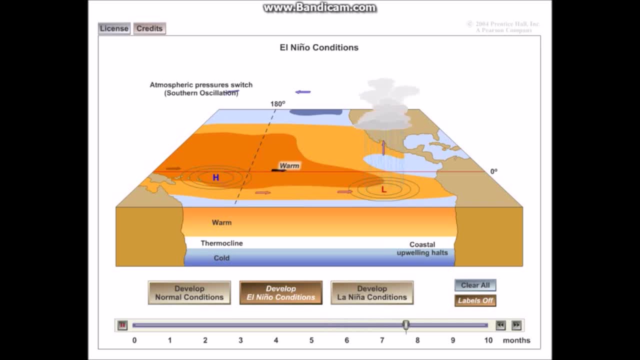 causes the precipitation to occur in the low pressure to occur off the coast of South America and it causes the high pressure and lack of rainfall to cross, to occur, sorry- of the coast of Southeast Asia. This, therefore, is going to cause a lot of flooding in Peru and 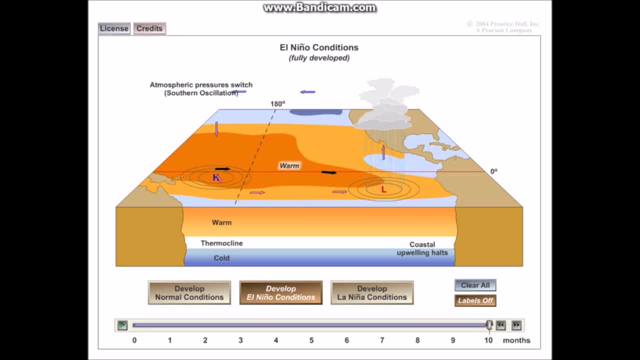 Chile and South America and potentially California, and is also going to cause droughts and therefore possibly forest fires in the rainforest regions of Indonesia and Darwin, North Australia and places like that. So, although El Niño is just a change of atmospheric and also water conditions in the Pacific Ocean, 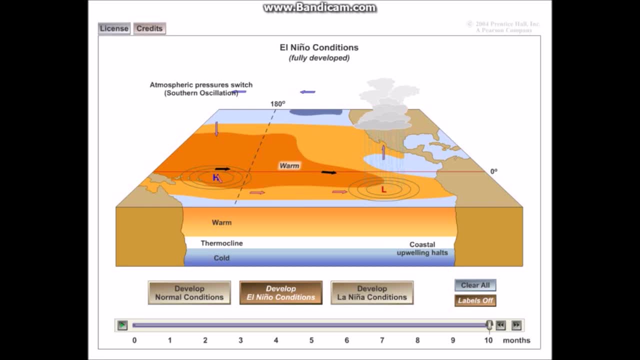 the. it has far-reaching effects all across the planet and has been blamed for potentially causing hurricanes or droughts in other parts of the world too, Nor because of this shift in or this oscillation in, atmospheric conditions and a change in sea level temperatures as well. 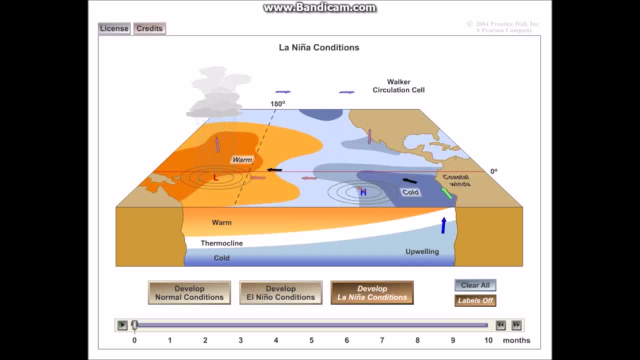 Finally we have La Niña. Now. on this map over here you can see that we have a normal conditions. currently. La Niña is kind of like a pendulum: You go from normal conditions to El Niño and after El Niño it tends to swing back towards normal. but sometimes that. 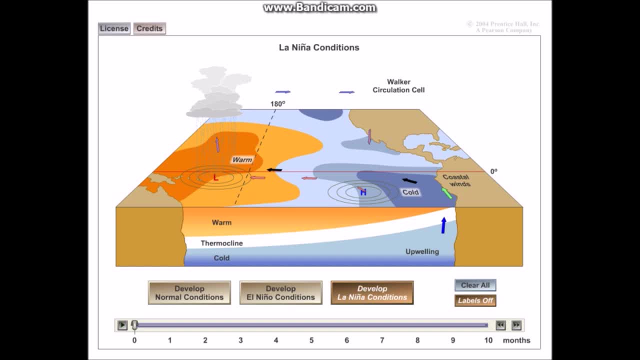 swinging back as a pendulum does, it overshoots and it becomes stronger than normal, and that's what La Niña is: It's a stronger than normal conditions. Now, if I start this video, you can see this. These are the normal conditions and these 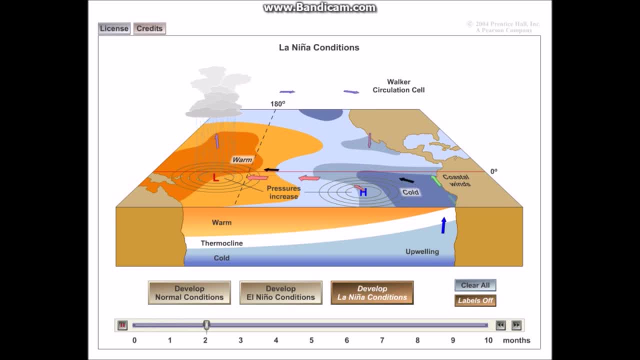 trade. winds actually become stronger and stronger and stronger, and as it becomes stronger these tend to move the area of low pressure further towards the land. and also these surface currents become stronger because the wind is also becoming stronger, The upwelling of water becomes more intense, The cold water that 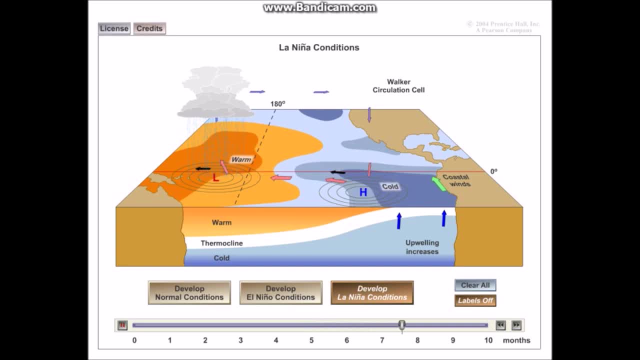 you have off the coast of South America begins to spread and to push itself towards Southeast Asia and typically what occurs is that the warm area becomes much warmer, You get a lot more precipitation and the cold area becomes colder and you get potentially more drought occurring in that area. 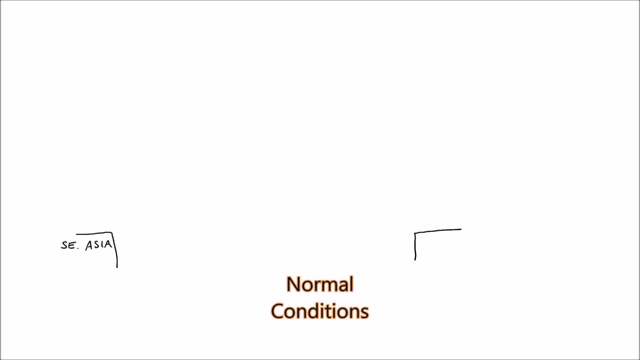 So, moving on to my hand-drawn diagrams, These are normal conditions. You have Southeast Asia, you have South America and you have to draw the Pacific Ocean. You start with the Walker Cell. You have the low pressure forming over Southeast Asia, you have the high pressure. 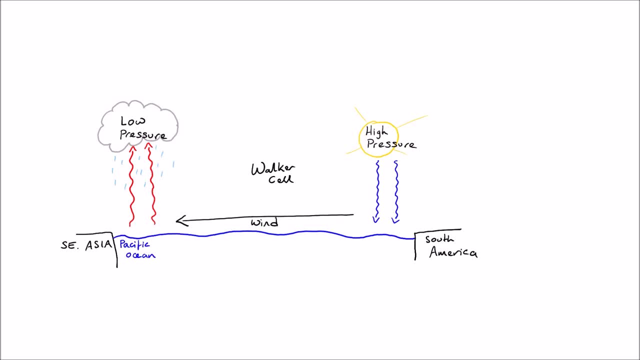 forming over South America and you obviously connect the two with the wind that is going to be blowing from high pressure to low pressure, That is going to cause the warm water to pull, even though there is currently a pretty well- publishing in the South East Asia- and the cold upwelling to occur in the South American. 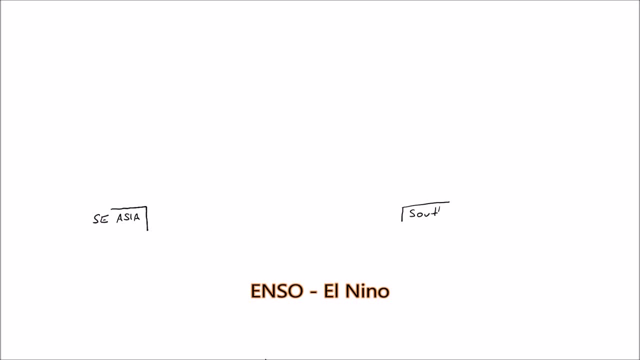 coast In ENSO conditions. on the other hand, the diagram is pretty much the same, other than the fact that you are going to be reversing the Walker cell. This is because the trade winds weaken, Obviously, as I said, the Walker cell. 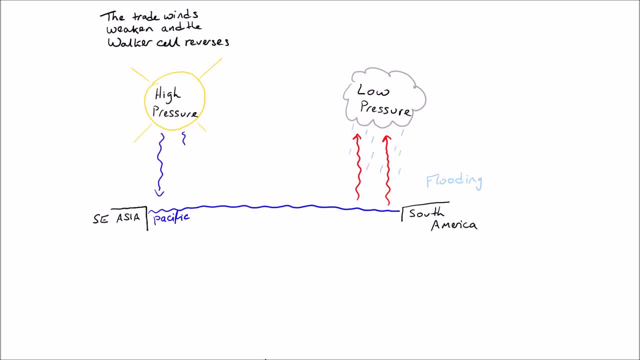 reverses. Low pressure is off of South America, causing flooding. high pressure is off Southeast Asia. It's going cause the winds to obviously move, if you the opposite direction, making warmer-than-normal conditions in South America and cooler-than-normal in Southeast Asia and causing drought there. Thank you very much for watching and have a really great day.